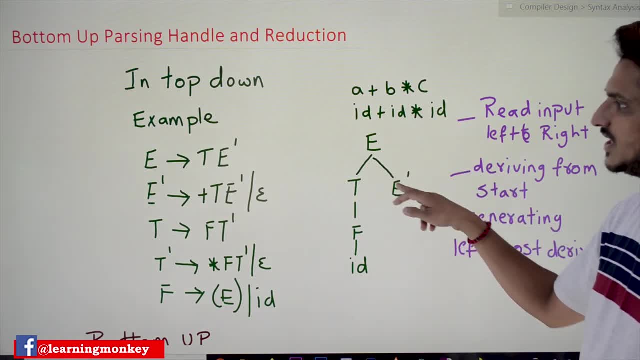 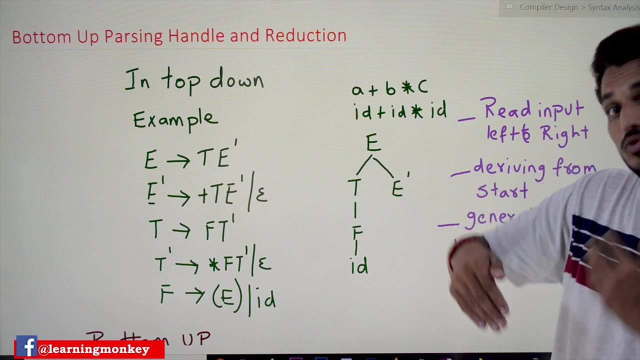 We are going to expand this: E. E is expanded as T, E, dash T is expanded as F. F is expanded as ID. The first ID symbol has been identified from the input. That is what we are doing. We are starting from E and we are going down towards to identify the identifier means, the input symbols. 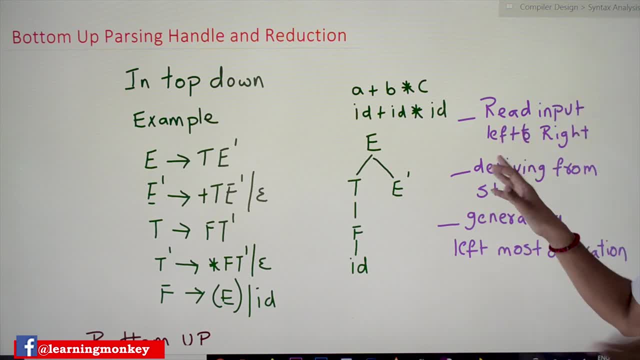 This is what we have done in top-down parsing. So the most important points are: read input left to right. In top-down parsing what we have done, We have read the input from left to right and we derived from the start symbol This is the start symbol. From start symbol we are going to derive that. 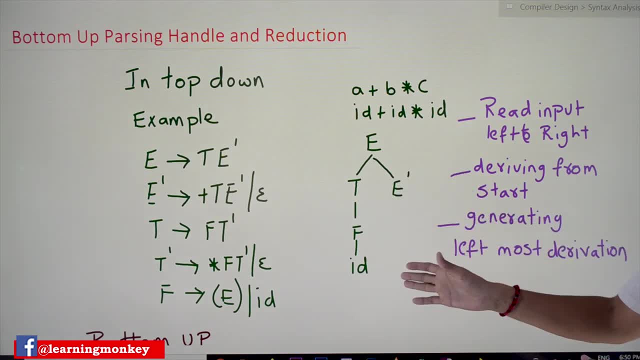 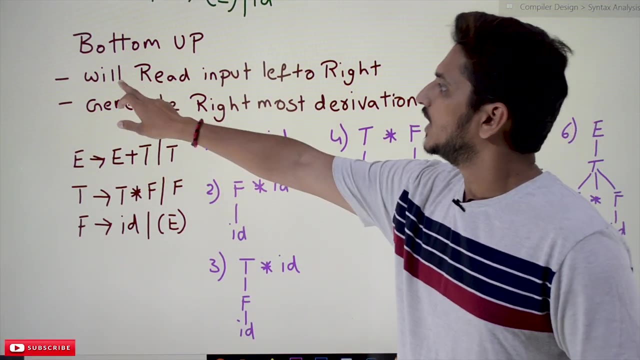 Next, we are going to generate left-most derivation tree. We keep on expanding these terms and identifying the left-most derivation tree. That is what we have done in top-down parsing, Coming to bottom-up parsing. What it will do here is it will read the input from left to right. 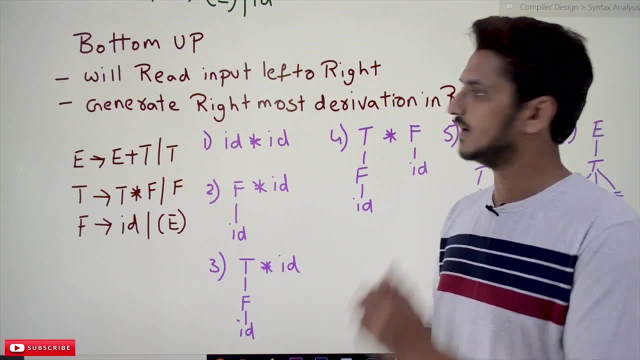 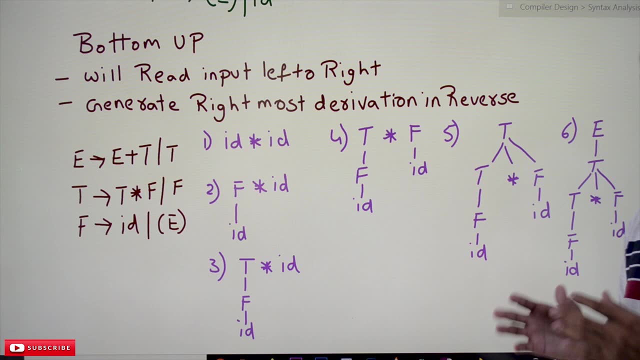 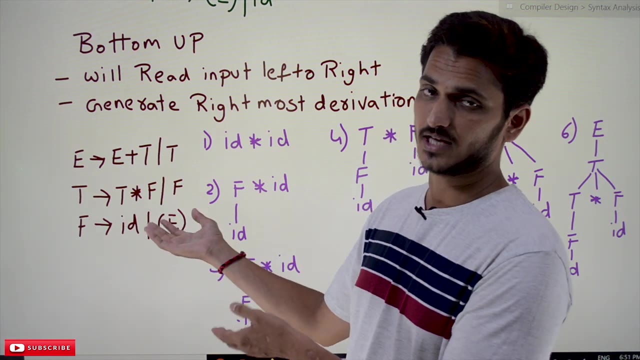 It is going to read the input from left to right, But it is going to generate right-most derivation in reverse. How it is going to generate, Let's try to understand step by step with an example. This is the example grammar which we are using to identify the expressions that consist of plus and multiplication symbol. 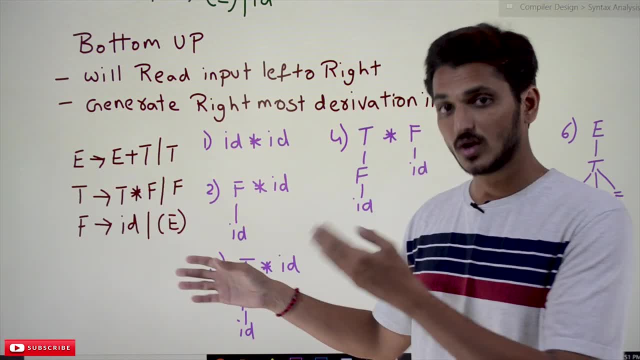 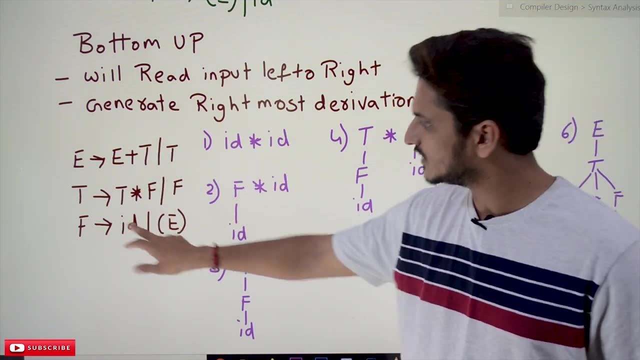 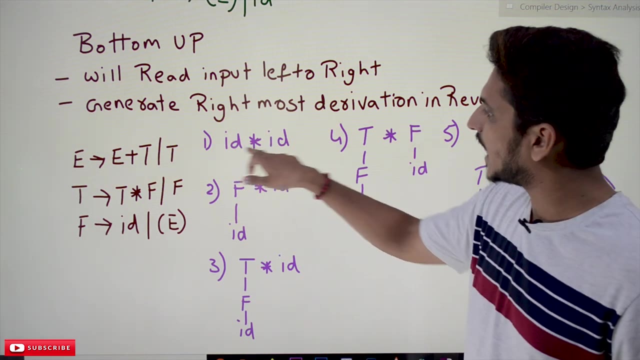 E tends to E plus T, T. These grammar were already discussed in our previous classes. That's why we are not concentrating on this grammar. T tends to T, star F or F. F tends to ID or bracket E. That is the grammar. if you want to identify the input: ID, star ID. 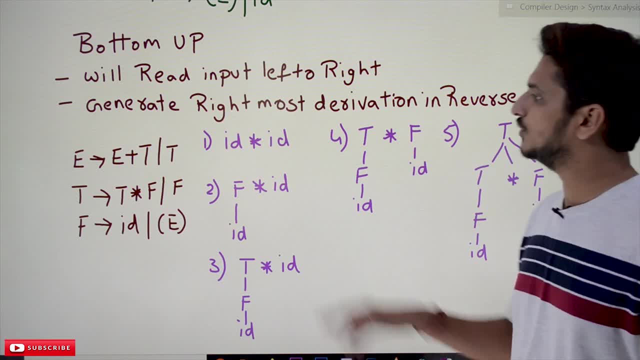 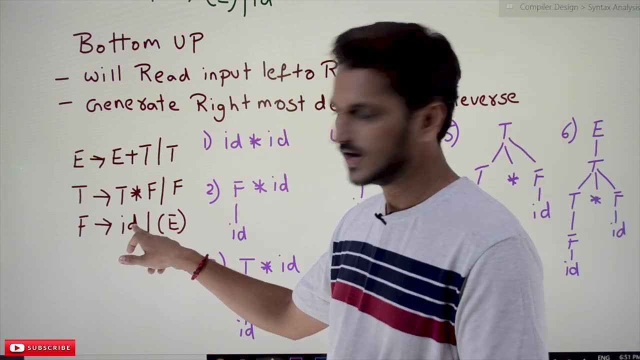 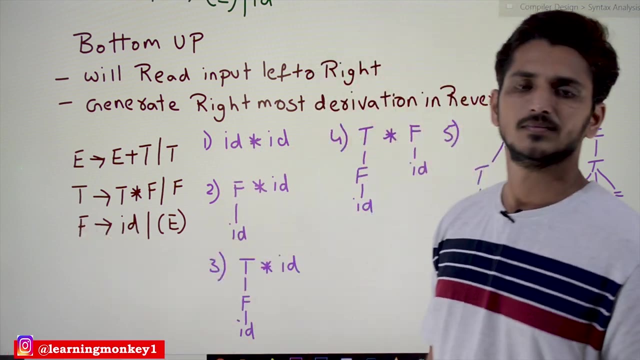 So what's bottom-up parsing is going to do? It will read the input from left to right. ID has been read. ID is identified as F tends to ID, So this ID is reduced to F. That's why it got the name reducing. 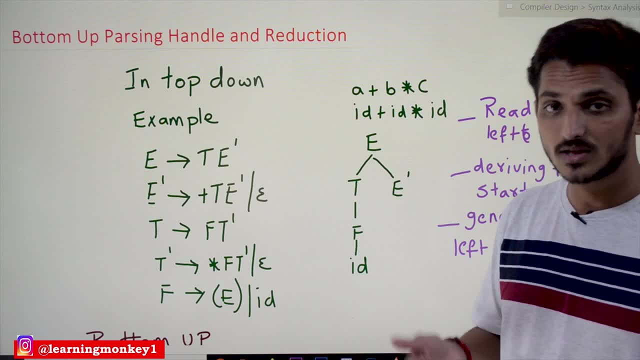 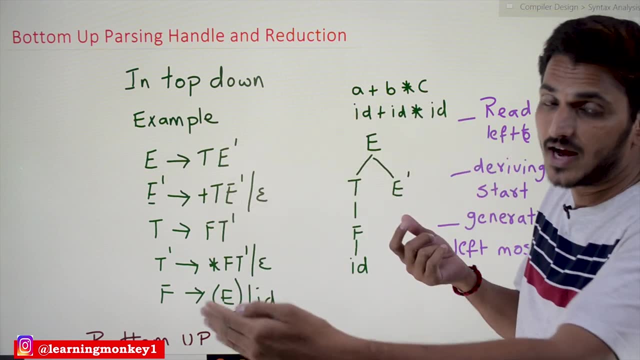 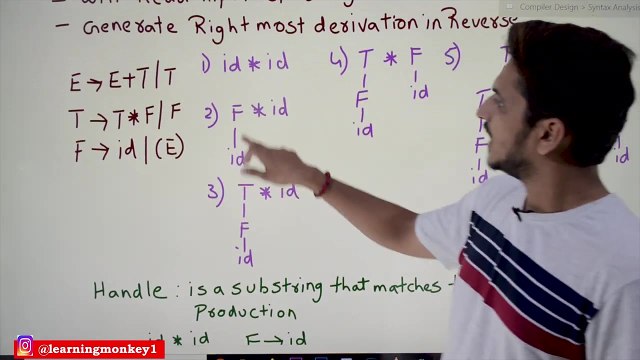 Reduction In bottom-up parsing. we are going to reduce the terms Check the input and reduce the term to the non-terminal that on the left-hand side of the production. That is what we are going to do. See, ID is reduced to F F- star ID. 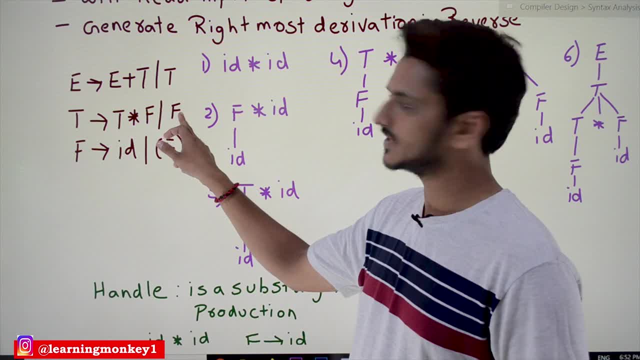 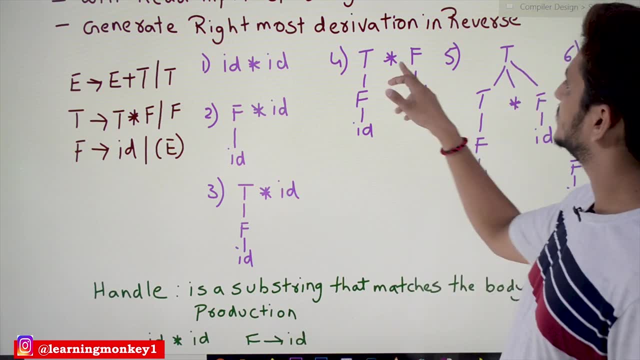 This is all. Next step, F, is on the left-hand side. F can be reduced to T. That's what happening here. F is reduced to T. Now next step is: this ID is reduced to F, So T, F, star, F ID. 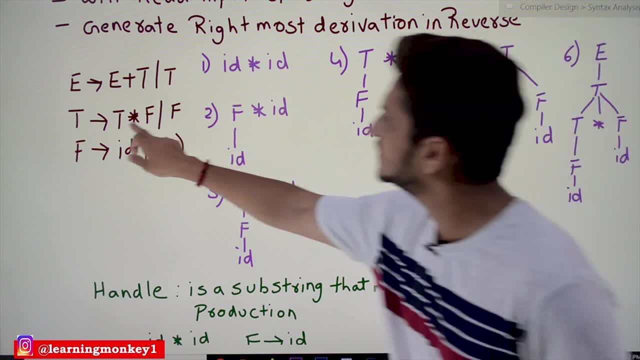 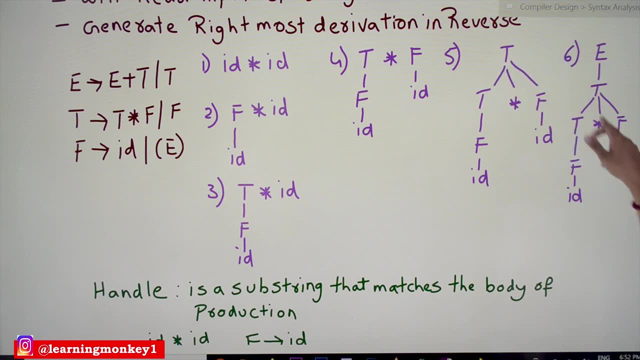 This is what we got. Now we are having T star F. T star F can be reduced to T. That is what happened in the next step: T star F has been reduced to T, And next we are going to have this: T is reduced to E. 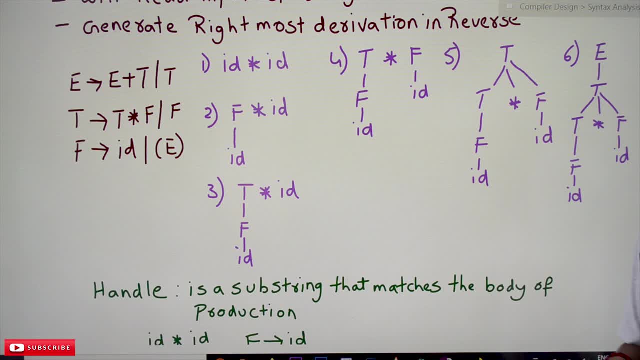 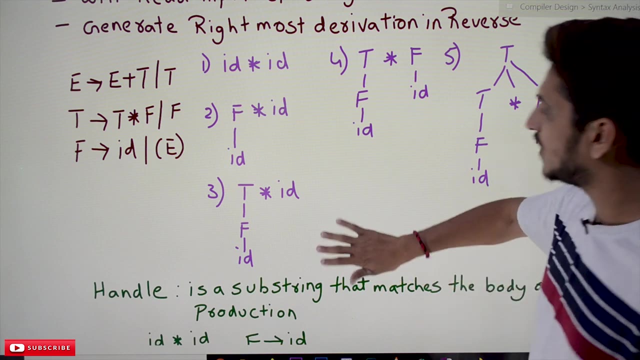 This T is reduced to E. This is how it is going to generate rightmost derivation in reverse. So bottom-up parsing is going to reduce the terms. In top-down parsing we are going to expand the terms. And one more important point you have to understand: 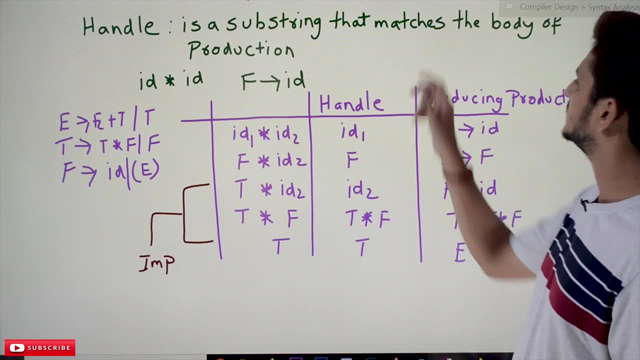 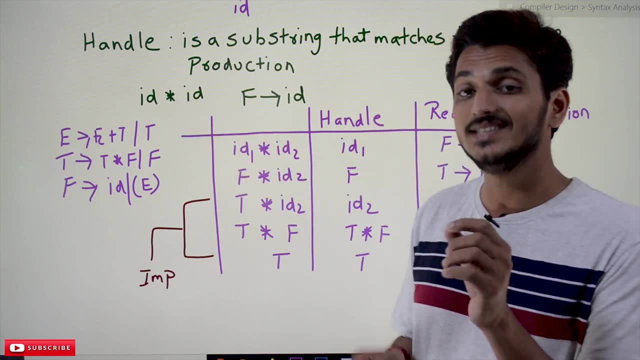 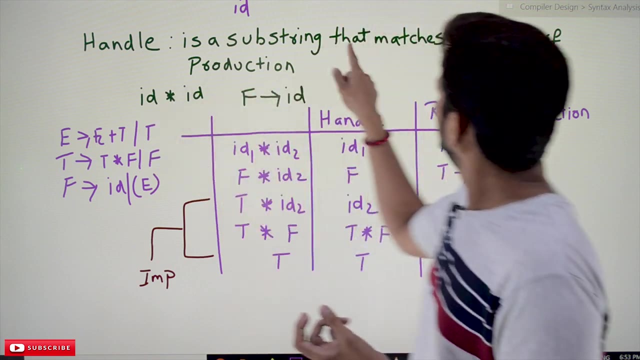 What is meant by handle Handle is a substring that matches the body of the production. Let's take the input ID, star ID. This is the input. Handle is a substring, So in the string it is going to be a substring If you take ID as a substring that matches the body of the production. 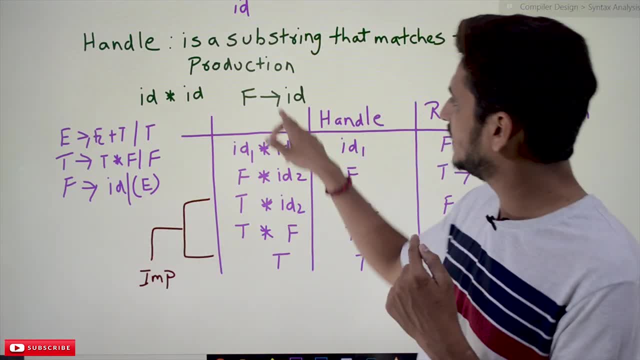 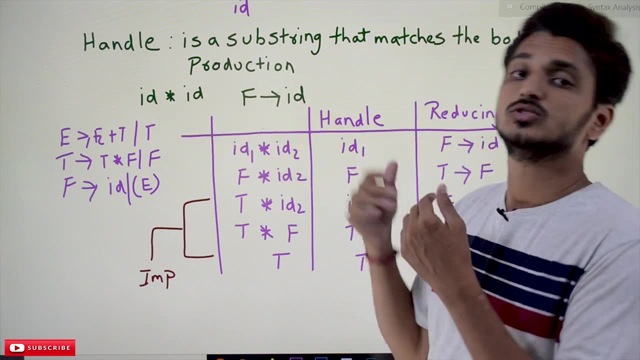 So ID is going to match the F tends to ID. If you take F tends to ID, what is the body of this production ID? So it is going to match the body of the production So that we can reduce that. That is what we call it as handle. 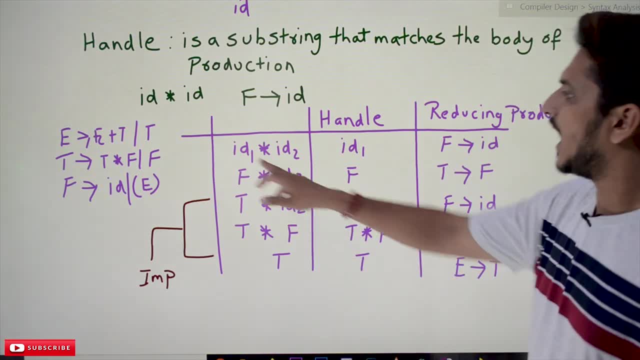 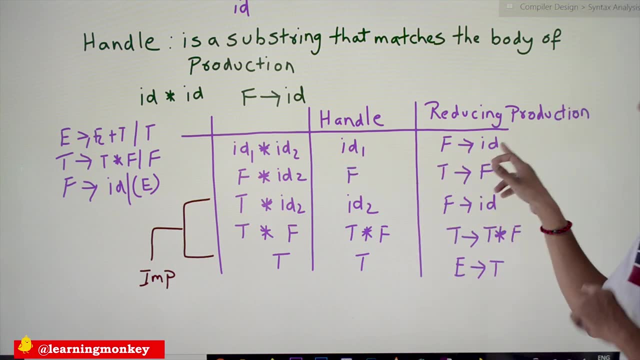 Okay, With this example you will get much clarity. ID star ID has been considered. What is the handle we considered here? ID1.. It is going to reduce ID1 to F, So next F star, ID2.. What is the handle we have considered here? 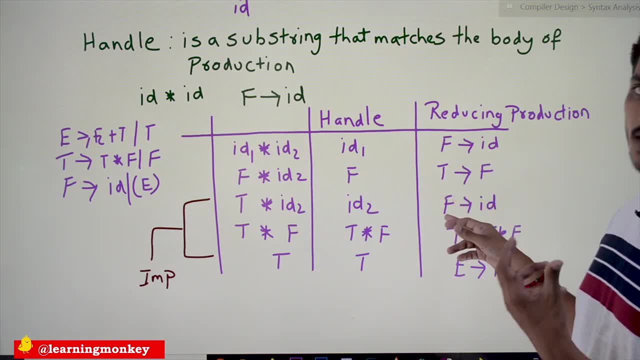 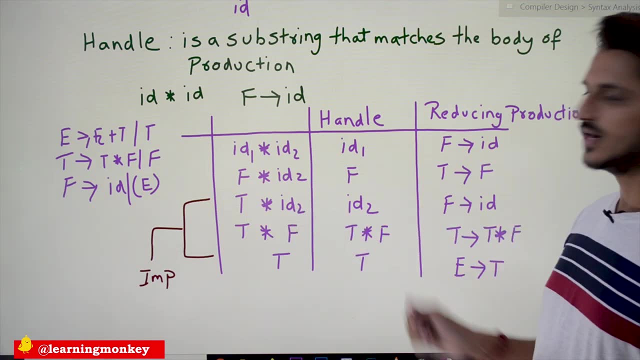 F. So what is the reduction production we have used here? T tends to F, F is reduced to T, T star. ID2 has been remained. What is the handle we have considered here? ID2 is considered as the handle. ID2 is reduced to T. 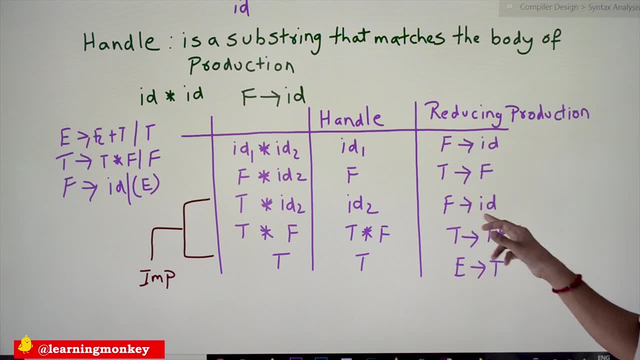 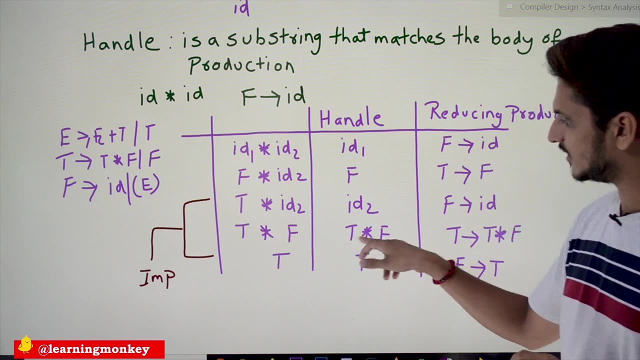 ID2 is reduced to F. That is why we used this production. Now, what is the T star F? What is the handle we have considered here? See here. This is the point: T star F. T star F is considered as handle. 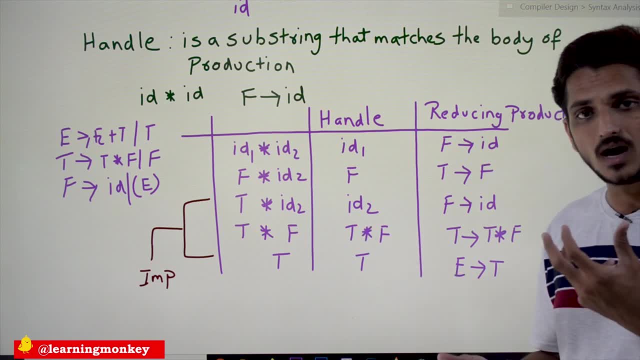 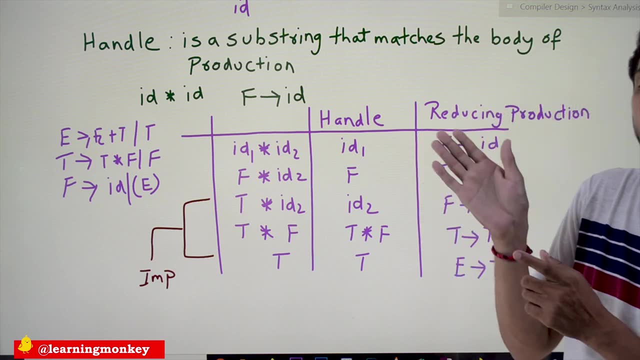 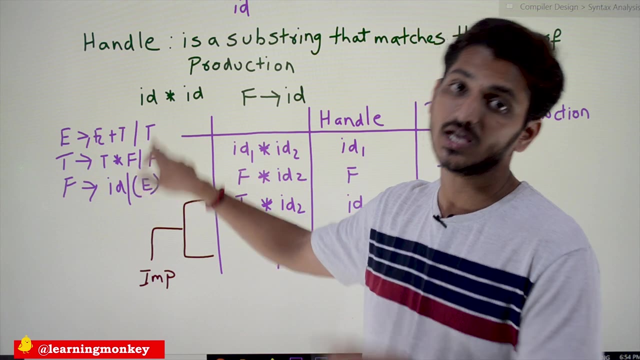 Because this is going ID handle is a substring that is going to be reduced. That match the left hand side production That match the body of the production. T star F That match the body of the production. This can be reduced to T. 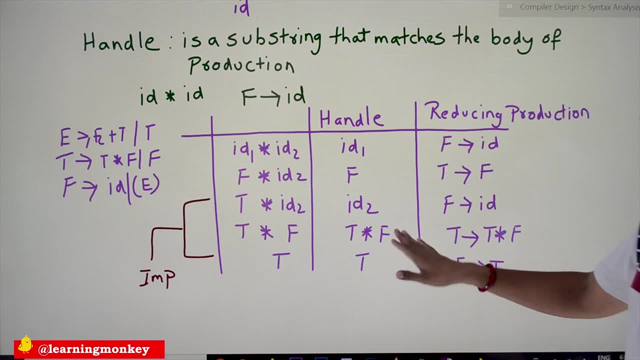 So T tends to T star F. Now T tends to T star F. What is remaining here T? What is the handle here T? So T can be reduced to E. Finally we got the start symbol. Means it is accepted. 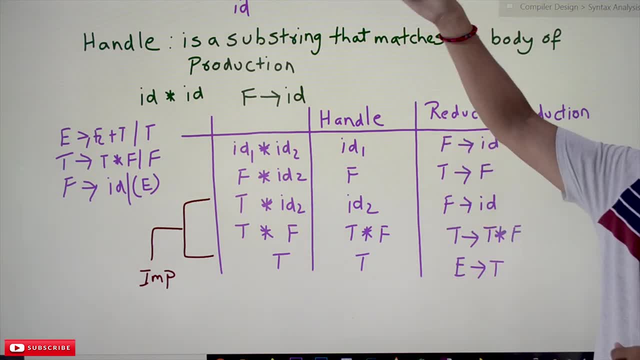 We are going from bottom to top. In top down parsing we are going from top to bottom. We started from E and derived the input string. Here we are taking the input string and reduce it to E. That is what we are doing in bottom up parsing. 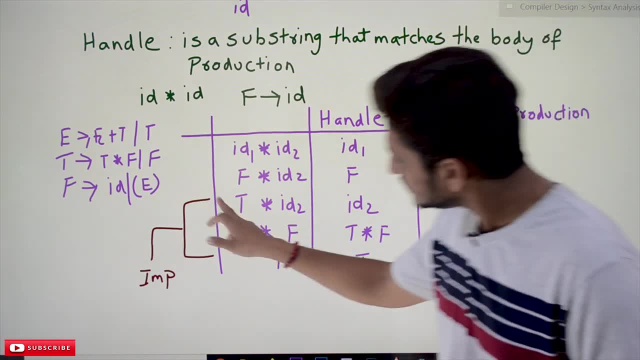 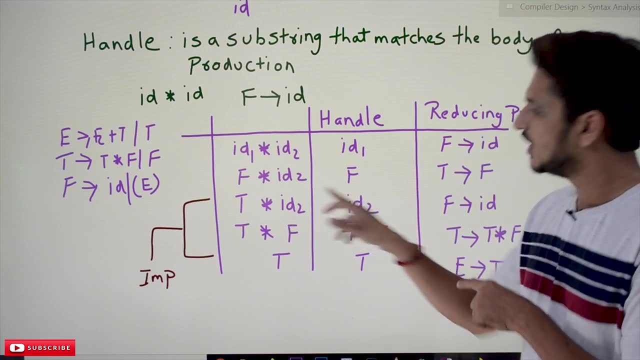 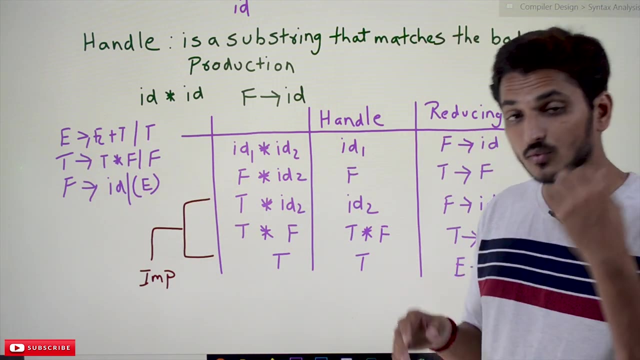 And one important point you have to remember here. See here, We have two options here: T star, ID. Why we considered the handle as ID to? Why not consider this: T can be reduced to E, T can be reduced to E, But we are not going to consider this T to reduce to E. 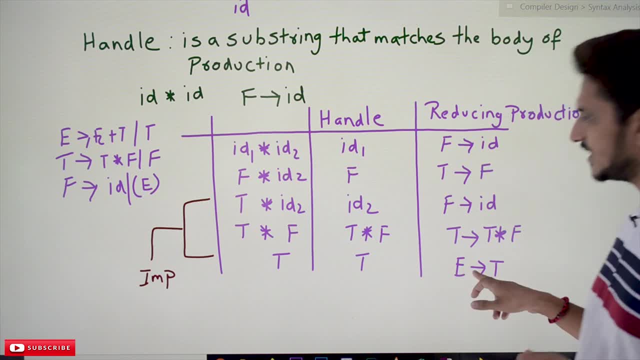 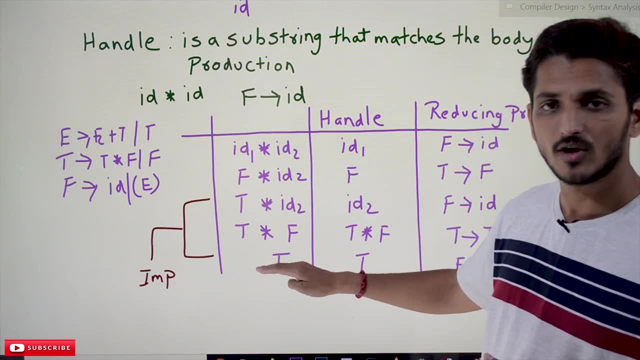 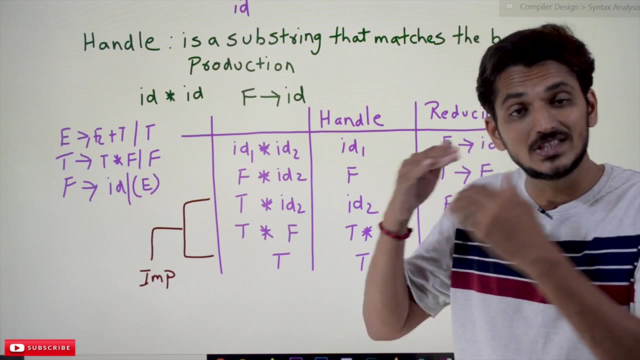 But here this T is considered as handle to reduce to E. But why we have not considered here Why we have considered this T as to reduce to E? This is the clarity we needed In which situations we have to take this to reduce to E. 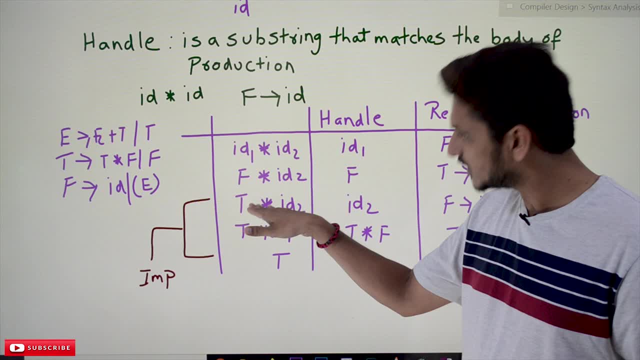 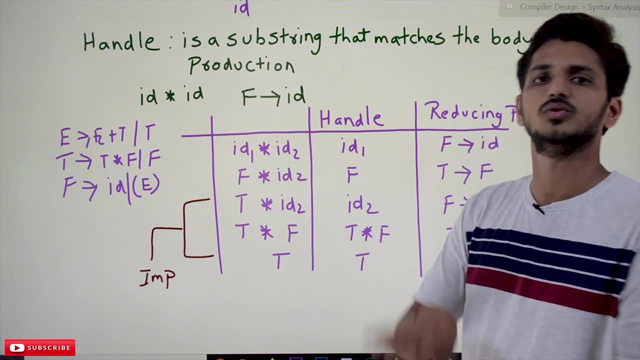 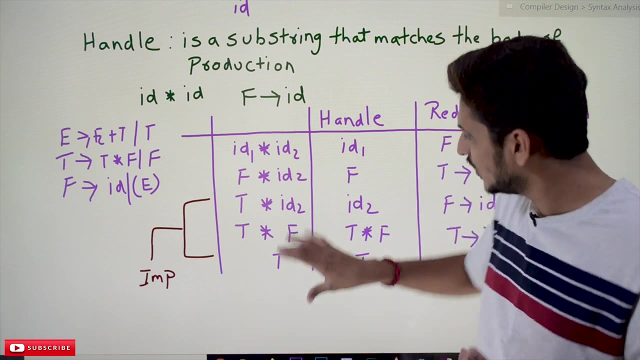 In which situations we should not consider T to reduce to E. In which situations we have to consider this T to reduce to E. This is the clarity we needed: How you get that clarity. In our next classes, we are going to identify the conditions. 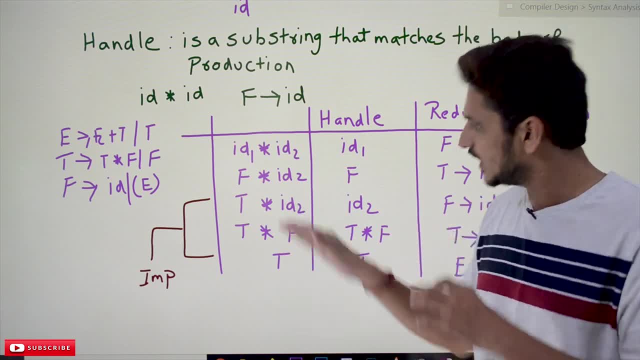 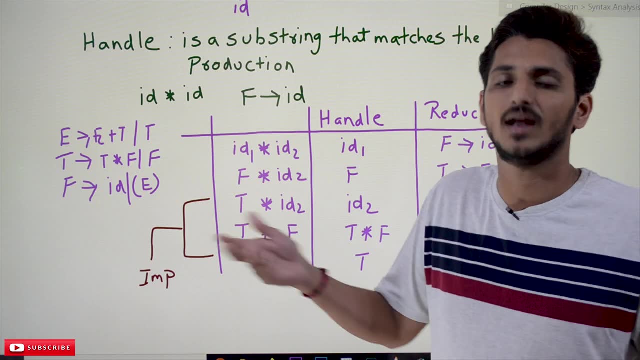 Where we have to reduce, Where we have to consider this handle, Where we should not consider this handle. That is the point we are going to understand in our coming classes. Hope you understand the concept. If you have any questions regarding the concept, 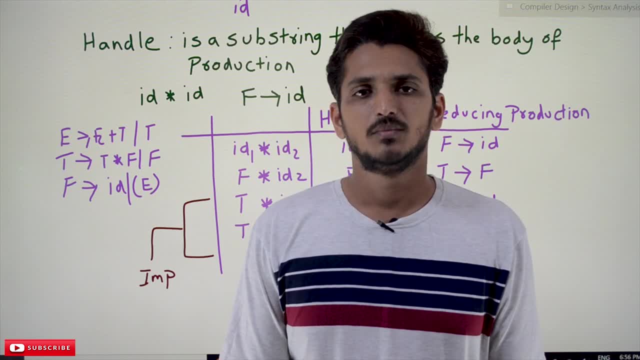 Please post your questions in the comment section. Please do subscribe to our channel and press bell icon for the latest update. Thank you.